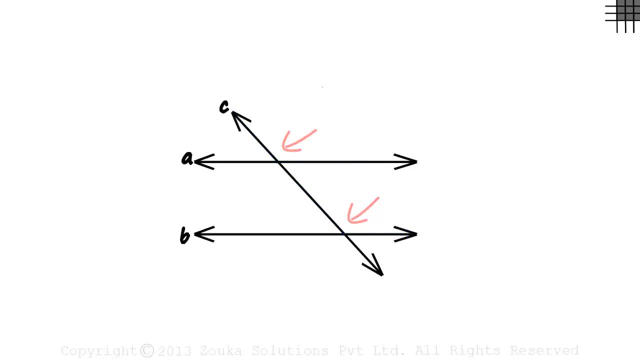 This tells us that the corresponding angles are always equal. Now let's go back to the previous page. Now let me ask you an interesting question. Look at the figure closely. Is this the only pair of corresponding angles? No, it isn't. 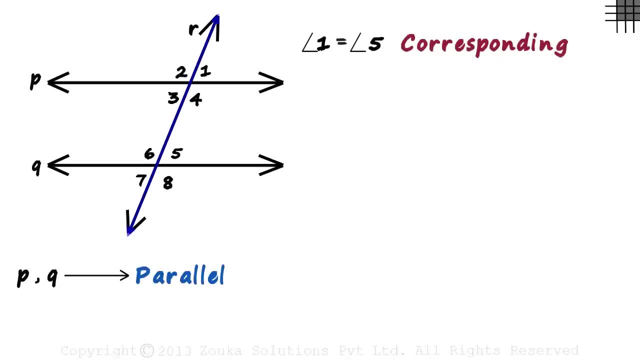 We have three more pairs of corresponding angles. When a transversal intersects a pair of parallel lines, four pairs of corresponding angles are formed. Two and six form a corresponding angles pair. So angle two will always equal angle six. You can even look at the figure and observe that they are equal. 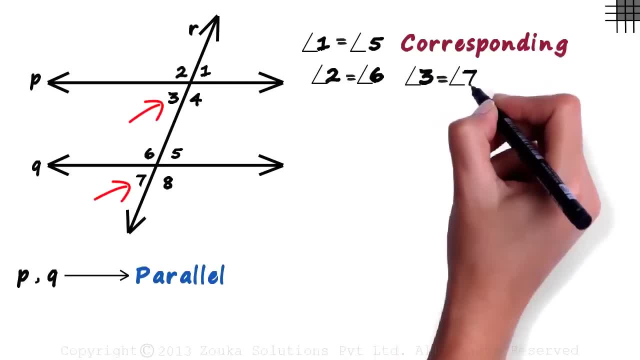 Similarly, angle three will equal angle seven and angle four will equal angle eight. These are the four pairs of corresponding angles that are formed: One and five, two and six, three and seven, four and eight. Angles three, four, five and six are interior angles. 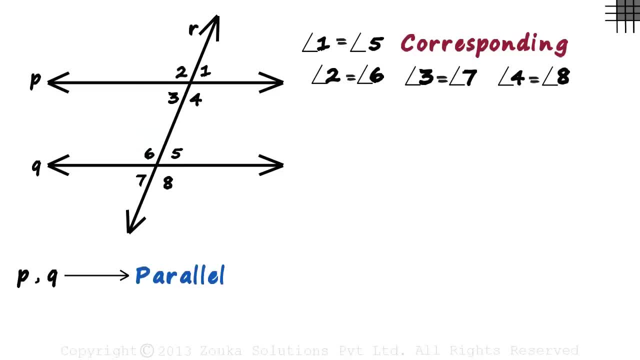 because they are between the two parallel lines And they are classified into two types. Let's understand the first type. Angle three and angle five form a pair of alternate interior angles. We know why they are called interior, But why exactly are they called alternate? 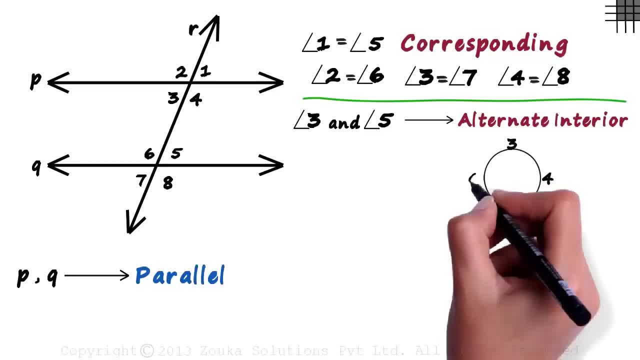 If we have a round table with numbers three, four, five and six around it, then five is alternate to three. That's because after three you skip one position and take the next. Similarly, six will be alternate to four. In this diagram as well, to find alternate of three. 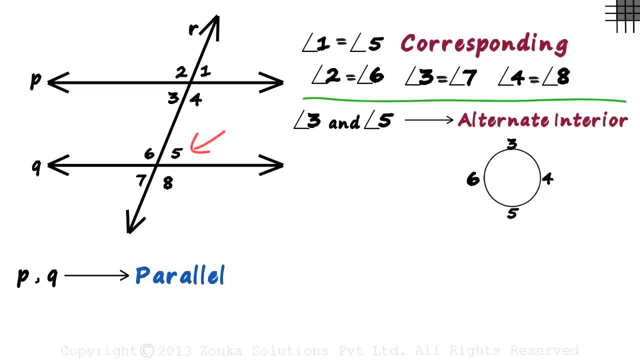 we skip one position and take the next, which is five. And similarly, angle four and angle six are also called alternate interior angles. This was the first type of interior angles. The second type is a pair in which the angles are next to each other on the same side of the transversal. 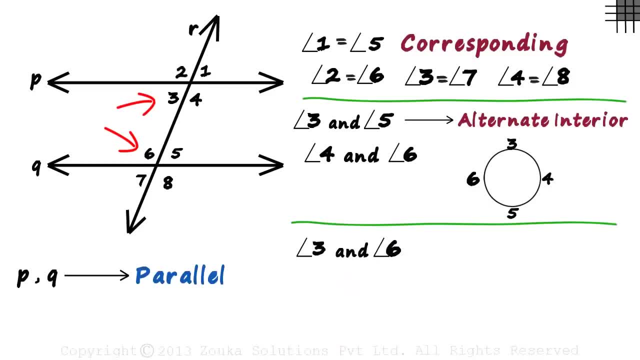 Like angle three and angle six, They are called consecutive interior angles. Look at the figure now. Do you see any other pair of consecutive interior angles? Yes, with the same logic, even angles four and five are consecutive interior angles. Remember, there are two types of interior angles. 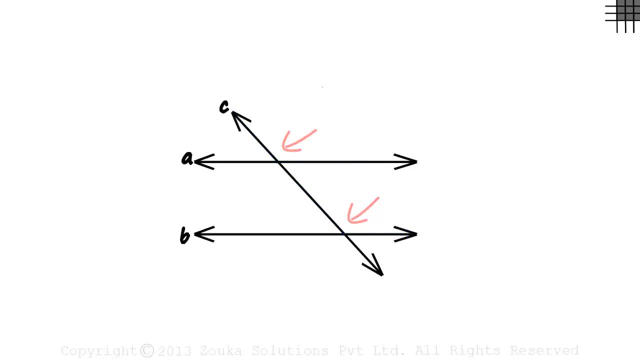 This tells us that the corresponding angles are always equal. Now let's go back to the previous page. Now let me ask you an interesting question. Look at the figure closely. Is this the only pair of corresponding angles? No, it isn't. 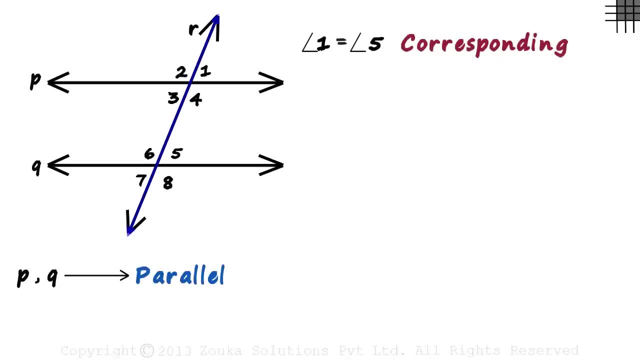 We have three more pairs of corresponding angles. When a transversal intersects a pair of parallel lines, four pairs of corresponding angles are formed. Two and six form a corresponding angles pair. So angle two will always equal angle six. You can even look at the figure and observe that they are equal. 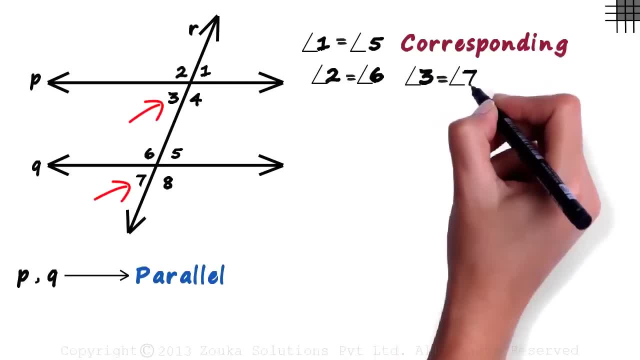 Similarly, angle three will equal angle seven and angle four will equal angle eight. These are the four pairs of corresponding angles that are formed: One and five, two and six, three and seven, four and eight. Angles three, four, five and six are interior angles. 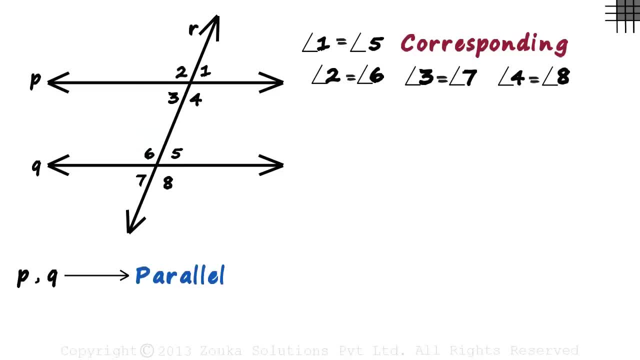 because they are between the two parallel lines And they are classified into two types. Let's understand the first type. Angle three and angle five form a pair of alternate interior angles. We know why they are called interior, But why exactly are they called alternate? 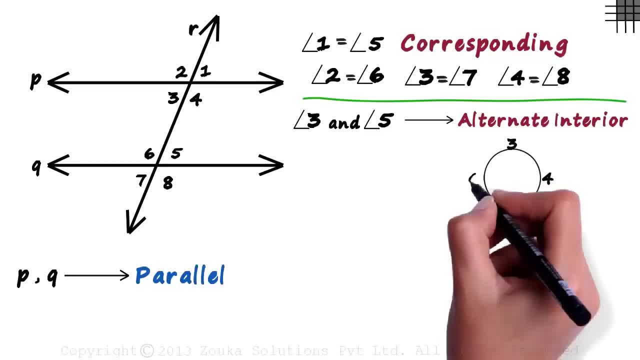 If we have a round table with numbers three, four, five and six around it, then five is alternate to three. That's because after three you skip one position and take the next. Similarly, six will be alternate to four. In this diagram as well, to find alternate of three. 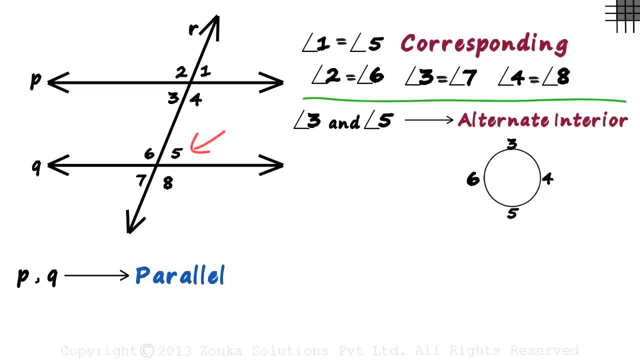 we skip one position and take the next, which is five. And similarly, angle four and angle six are also called alternate interior angles. This was the first type of interior angles. The second type is a pair in which the angles are next to each other on the same side of the transversal. 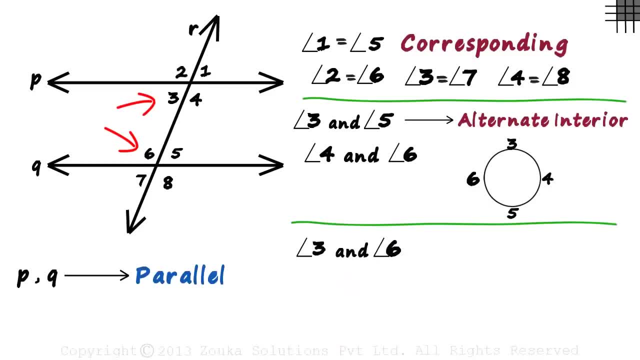 Like angle three and angle six, They are called consecutive interior angles. Look at the figure now. Do you see any other pair of consecutive interior angles? Yes, with the same logic, even angles four and five are consecutive interior angles. Remember, there are two types of interior angles.